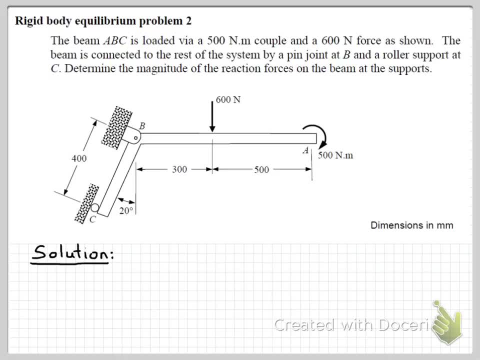 our solution. And as with virtually every engineering mechanics problem, the first thing we do is to draw a free body diagram of the component that we're trying to analyse. So in this case we're looking at the reaction forces on the component ABC. so we'll draw 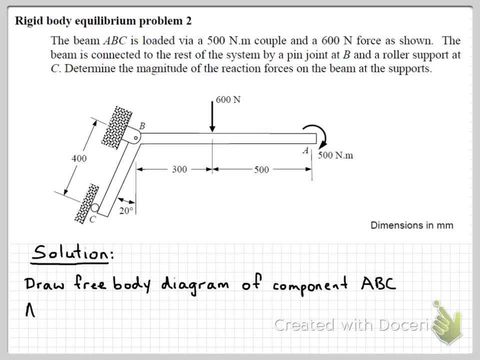 a free body diagram of that component. Next, this component is in equilibrium, so we'll apply the equations of equilibrium and then, of course, we'll solve those equilibriums for our unknown reactions. Okay, so let's go ahead and draw the free body diagram. 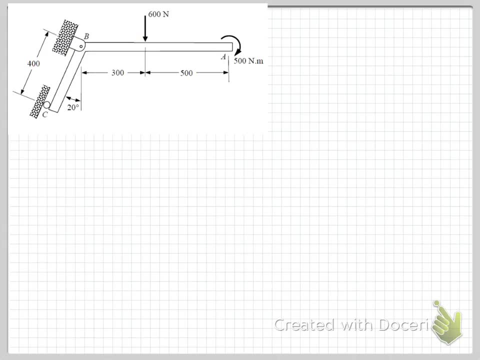 So I've just copied over the question here, question figure, so we can refer to that in drawing a free body diagram. So our free body diagram is simply an external, or the representation of the external extremities of the body that we're analysing. Okay, so in this case it's. 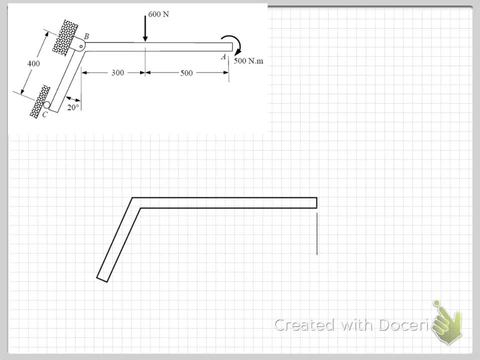 just our simple shape like this, And then, once we've got that, we can start adding in some of the more important dimensions. You don't need to do that. You don't necessarily need to include all of them, but the most important ones for calculating. 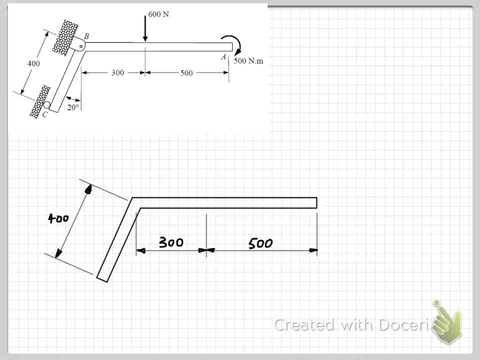 the moments and some of the angles you should have. Then we'll also go and label the important points. so ABC, the end A where the moment is applied, and our two support points. Okay, I notice, I haven't put in the angle there. 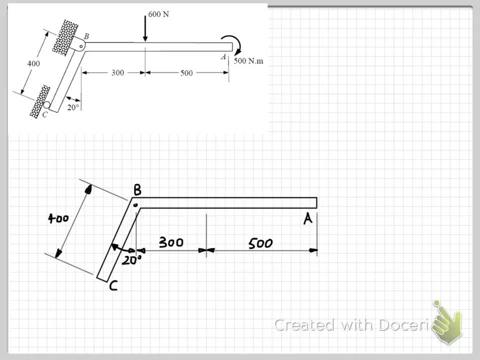 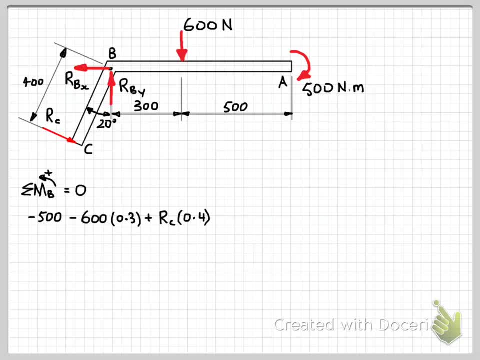 Okay, so to be consistent in our units, we've got newtons here, so our distances here will have to be in metres. So then of course that's all equal to zero. So note how the equation of equilibrium is written. 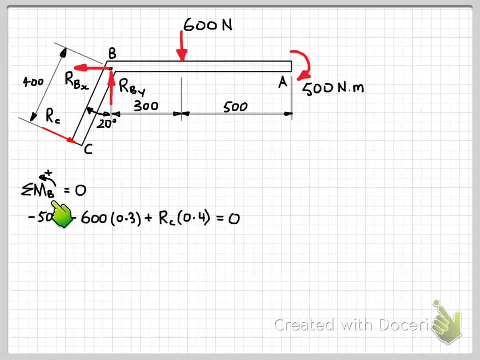 So we've got some of the moments, some of the moments Here. we have some of the moments about point B And we've noted that we can now check that we've used the correct distances in writing this moment equation because we know we can look here. okay, moments about point B. 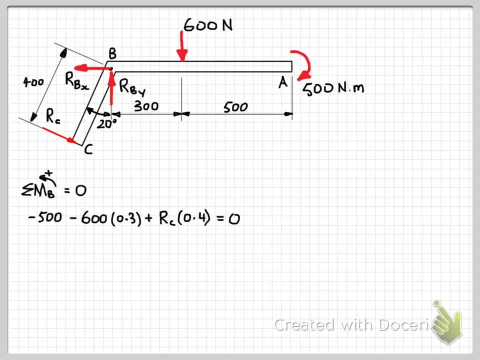 We can go back up to our diagram and check those distances And then all of our moments are equal to zero. Okay, so some of the moments equal to zero. So that gives us our equation that we can solve for our one unknown RC. and if we just do the maths there, quite simple. 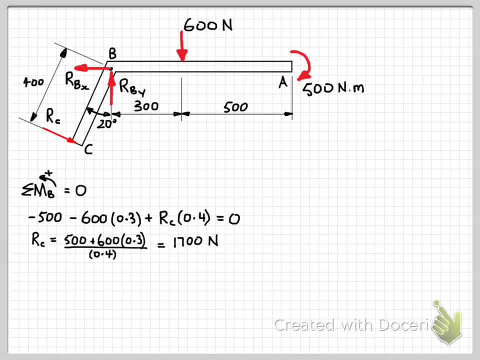 Rearrange the equation and we get a force of 1,700 newtons. Also, remind you that the moment couple here is a free vector. We could apply that anywhere on the beam or the component and it would have the same external effect on the body. 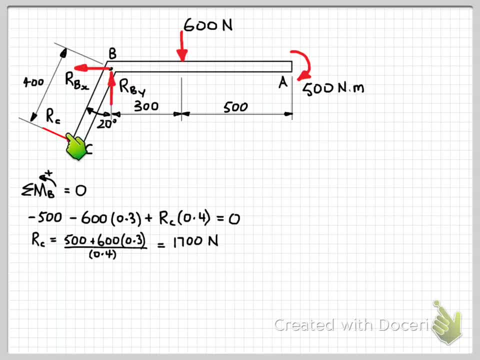 ie our reaction forces that we calculate here and here would be equal to zero. So it's exactly the same, no matter if we apply the load here as it's shown or if we apply the moment here, for example, And you can see that also in the equation. 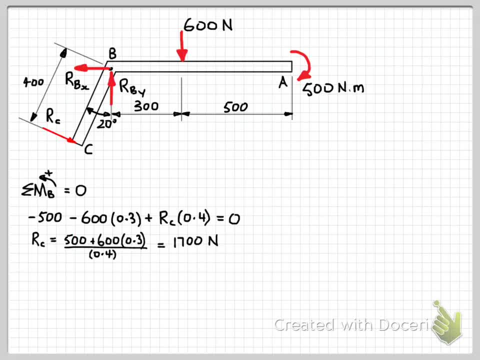 There's no distance associated with this moment. Okay, Also, look at the units. So this is in newton meters. So if we multiply this by a distance, then we'd have newton meters squared, which then of course means that we have inconsistent units in our equation. 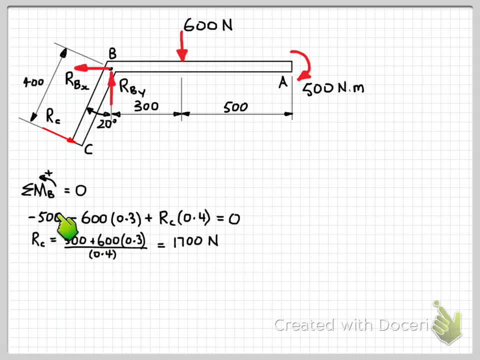 Okay. So I see a lot of people make mistakes with applying this moment here. So just think about those things and hopefully that will stop you or help you- help prevent you- from making those sorts of mistakes. Okay, So now that we have that, we can apply our other equations of equilibrium. 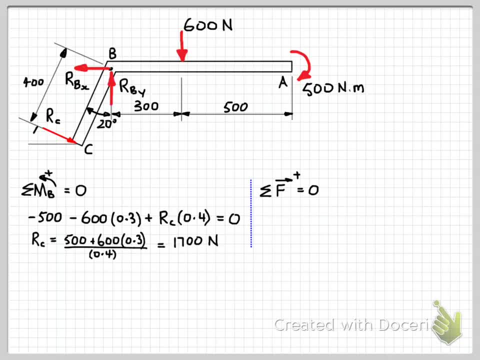 So let's start with. sum of the forces in the horizontal direction equals zero, And in this case, if we look up here, we've got RC acting at an angle 20 degrees to the horizontal. So what I'm going to do here is to just calculate the. 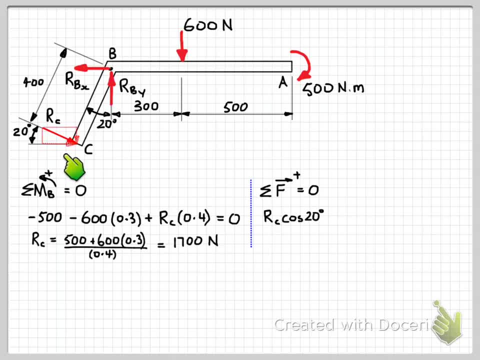 or use the components of that force in the horizontal and vertical direction. So here RC cos 20 degrees will be our horizontal component, And then our only other horizontal force in this problem is our reaction, RBX. Okay, Again in our equation of equilibrium. 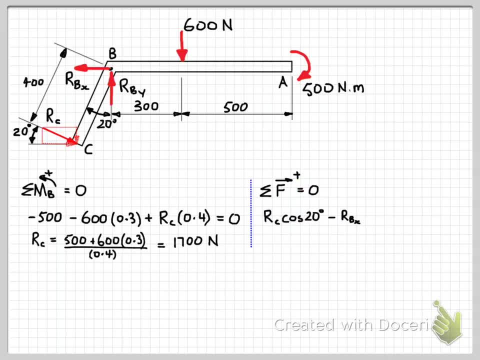 sum of the forces. Here we've got: sum of the forces equals zero. So our correctly written equation will look like this: Here are our forces. Adding them all up, and they are all equal to zero. gives us an equation that we can now solve for RBX. 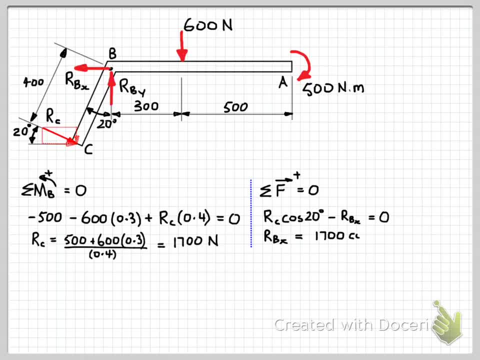 because we've just calculated RC. So if we go ahead and do that we'll get just by rearranging the equation again, and we get RBX equals 1000.. So that's 1597.5 Newtons. All right. 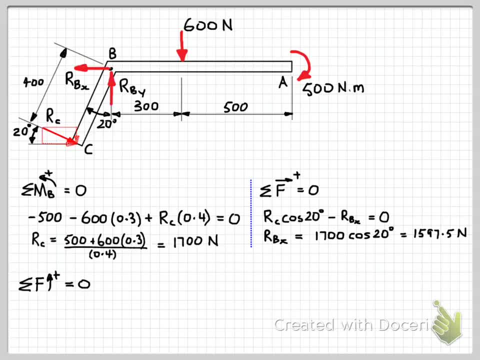 Now let's apply our third equation of equilibrium: sum of the forces in the vertical direction equals zero. So again we have the vertical component of our force, RC. So in this case RC sin 20 degrees And it's in the negative direction, so acting downwards. 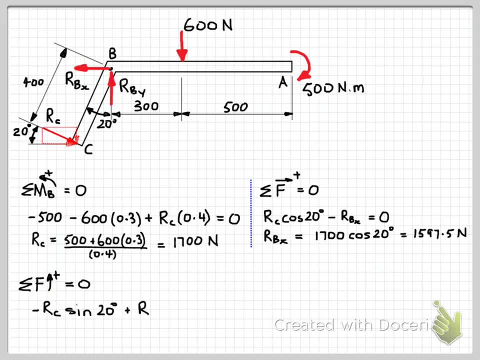 And we've indicated here that positive is upwards. We also have RBY, which is our only remaining unknown, and our 600 Newton applied load, Again, sum of the forces all equal to zero Again, do your algebra rearrange the equation?